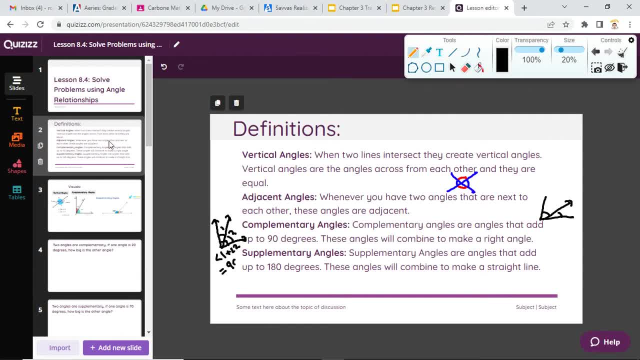 angle one plus angle two will be equal to 90 degrees. The last one I have is supplementary angles. So supplementary angles are angles that add up to 180 degrees and they combine to make a straight line. So if I have a right angle, I have a right angle and I have a right angle. 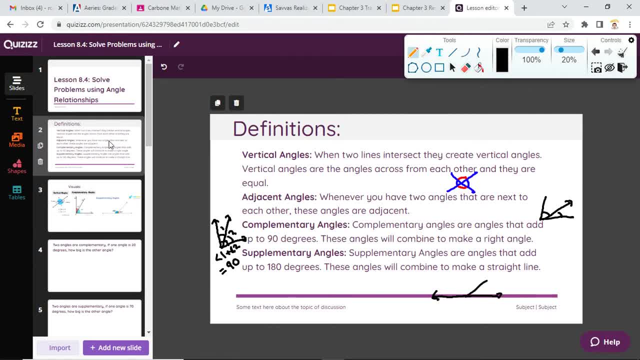 and I have a right angle. I have a right angle and I have a right angle and I have a right angle. If I look at a line like this here and it's broken up into two parts. let's call this angle A and angle B. 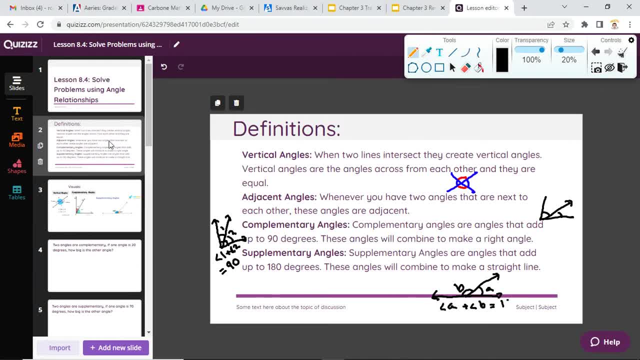 I can say that angle A plus angle B will be equal to 180 degrees. Alrighty, those are our definitions today. If you guys need, to make sure to get these down here and you do pause your video so you'll be able to. 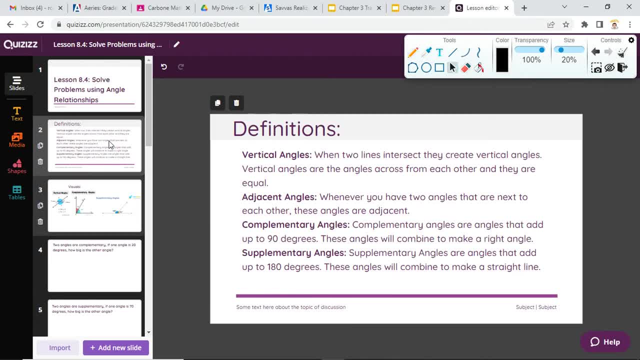 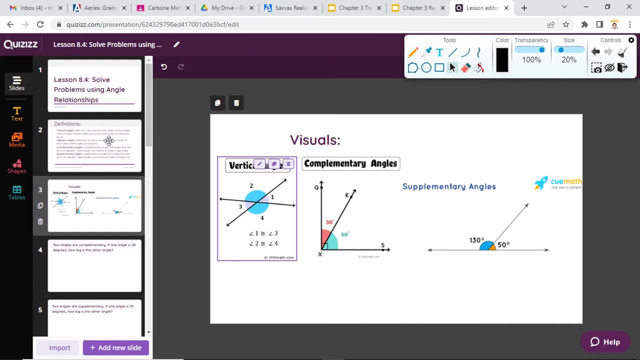 I'm going to move forward here, Alright. so I want to give you guys some visuals to look at these here. So the one on the left: here are some vertical angles. What we can see is two lines intersecting, and then I have four different angles: angle 1,, 2,, 3, and 4.. 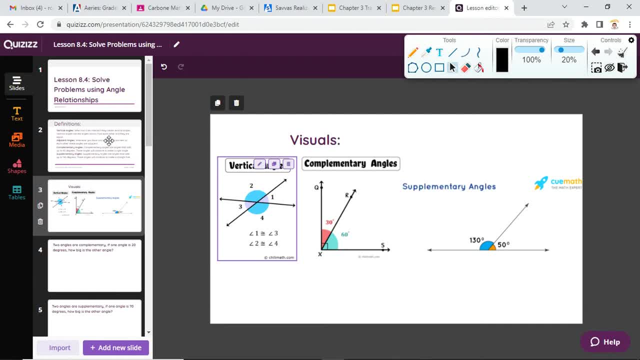 And we have to look at the ones across from each other and those are going to be our pairs of vertical angles. So it turns out angle 1 right here is congruent, or the same as angle 3.. Angle 4 right here is congruent, or the same as angle 2, meaning they have the same angle measurements. 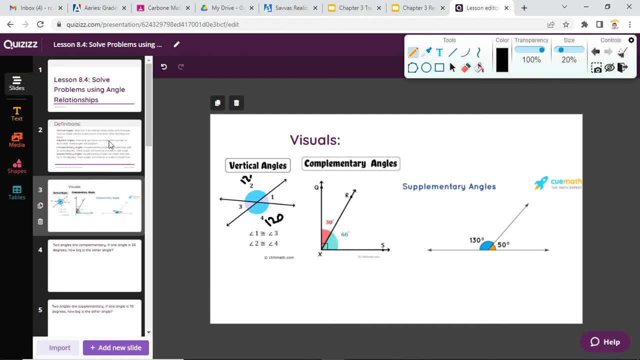 So if angle 4 was 120 degrees, angle 2 would also be 120 degrees. If angle 1 was 60 degrees, angle 3 would also be 60 degrees, To our right. here we see a pair of complementary angles. 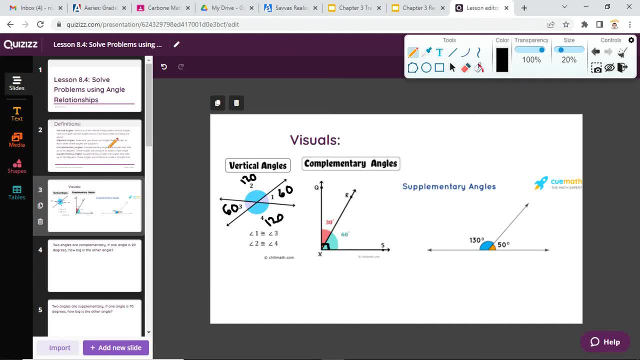 So notice how I have a right triangle down here, or, excuse me, a right angle down here in the bottom right. That means that this total angle right here is 90 degrees. And notice the two angle measurements inside. I have a 60 degree angle and a 30 degree angle. 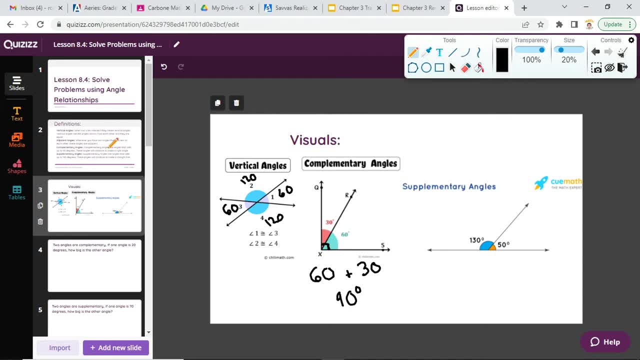 If I add those together, 60 plus 30 is 90 degrees, because those two angles are complementary. Last one we have here is supplementary. Supplementary are two angles that add up to 180 degrees. right, They form a straight line. 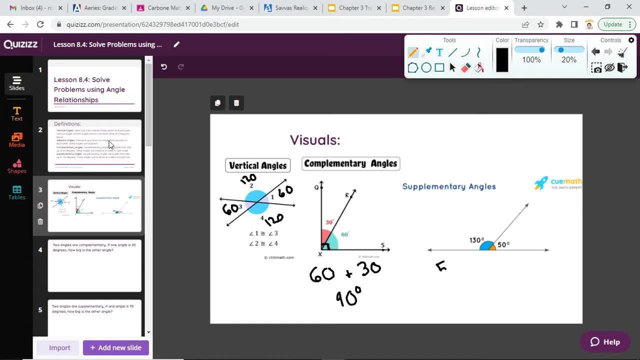 Notice. this is my straight line here on the bottom and then my two angles inside. I have 50 degrees and 130 degrees And if I add those together- 50 plus 130, I get 180 degrees because those two angles are supplementary. 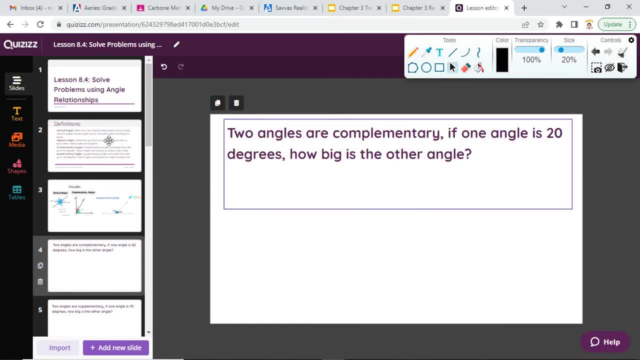 Alright, so two angles are complementary. If one angle is 90 degrees, how big is the other angle? Alright, so what I want you guys to remember is: when two angles are complementary, that means angle 1 plus angle 2 is equal to 90 degrees. okay. 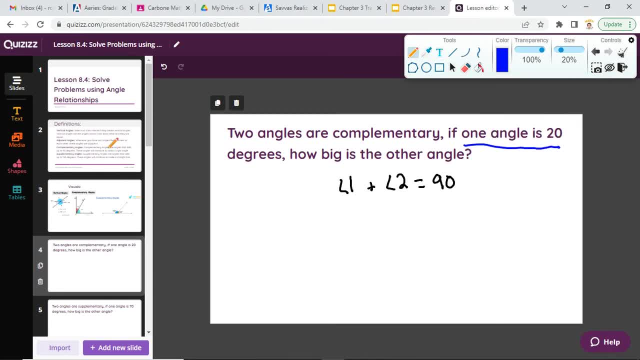 Here it tells me that one angle is 20 degrees, so I'm going to place angle 1 here with 20 degrees. So 20 degrees plus angle 2 is equal to 90 degrees. Well, the opposite of adding 20 is subtracting 20.. 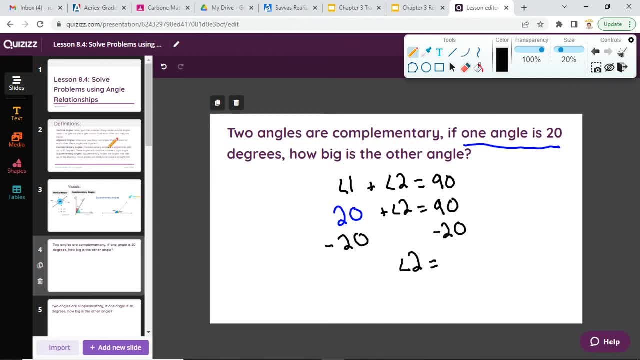 We've got to do that on both sides here, so I get: angle 2 is equal to 90 minus 20 degrees, 70 degrees. Now, that's if you want to solve that algebraically, which is the way I like to solve these problems. 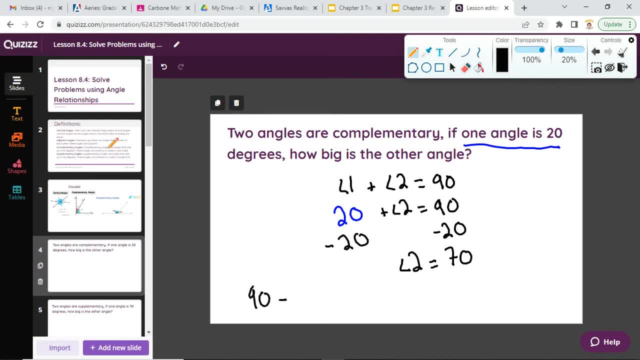 However, yes, on this problem, you could have just taken your 90-degree angle and subtracted the one angle you knew. 90 minus 20 is 70 degrees. However, I like to do it algebraically, because we have a clear explanation of everything that's happening. 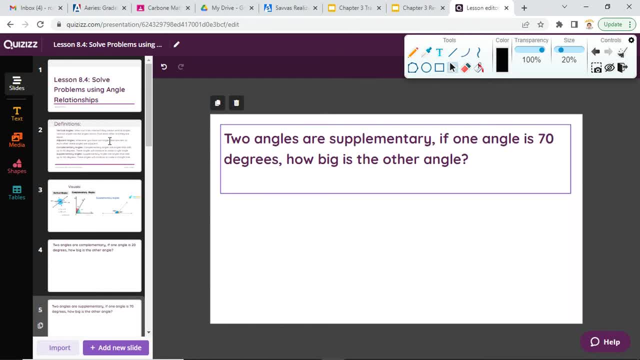 Okay, next question. here, Two angles are supplementary. If one angle is 70 degrees, how big is the other angle? Again, since they are supplementary, that means they form a straight line, right? It's going to look like this: 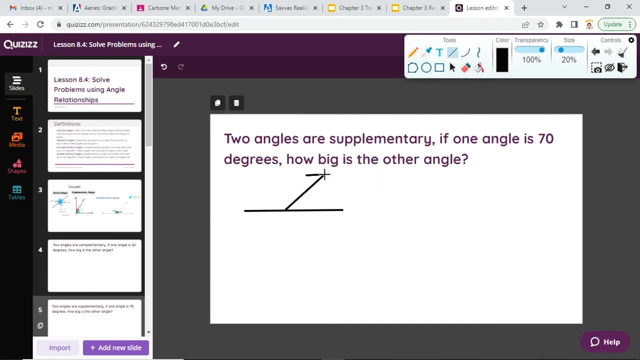 Okay, that's why I have oopsie-daisy. I don't want that to be there. I have one angle that is 70 degrees and I've got a question mark for my other angle. Remember, they're supplementary. 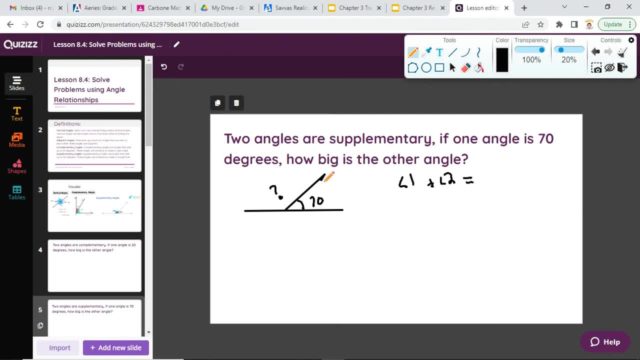 That means angle 1 plus angle 2 will add up to how many degrees? 180 degrees. Alrighty, here it tells me one angle is 70 degrees, so I'm going to replace angle 1 here with 70 degrees, So I have 70 plus angle 2 is equal to 180 degrees. 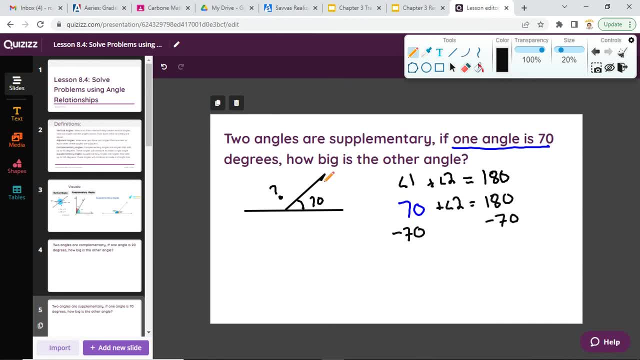 Well, it's the opposite of adding 70, but subtracting 70,. we'll do that from both sides and we get that angle 2 is equal to 110 degrees. Again, that's how to solve it algebraically. Yes, you could have done the logical step of doing 180 minus 70, which is equal to 110.. 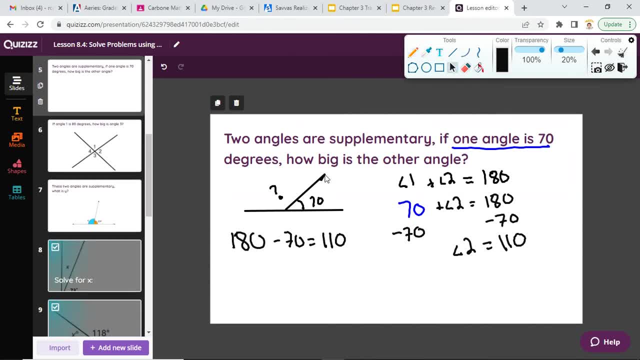 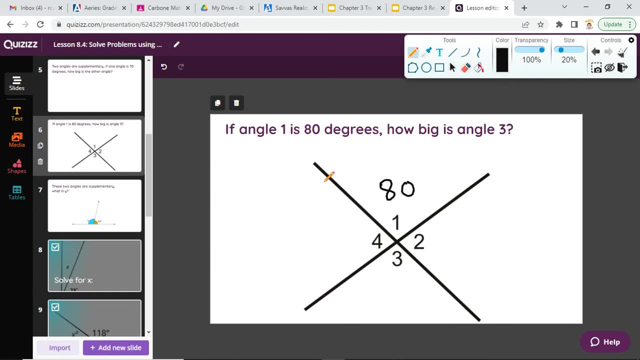 All right, a couple more examples for us here. If angle 1 is 80 degrees, this angle right here is 80 degrees. how big is angle 3? Angle 3 right here. So notice what we have. We have two intersecting lines.